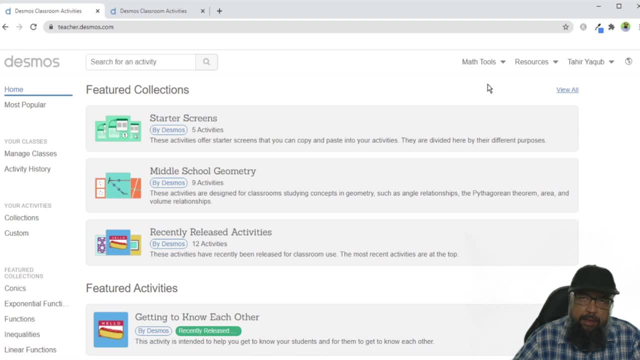 by using their Google account, And now I have logged into my Desmos account as a teacher. So first let's have a look at some of the math tools available. As you can see that there are various math tools available, I have made other videos about math tools which you can watch, And 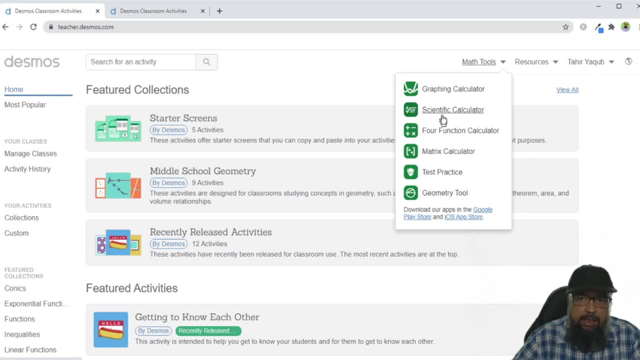 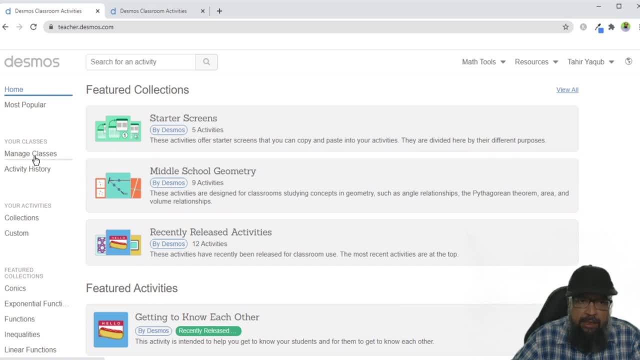 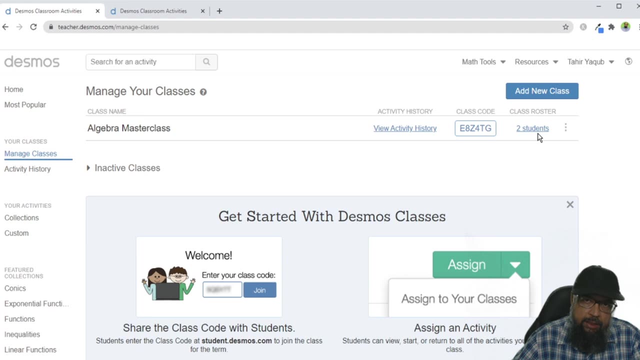 do math activities. I have to click on manage classes on the left hand side. If I click there, I have only one class at the moment in which there are two students And basically I have joined this class by using two other devices. And let us see how you can. 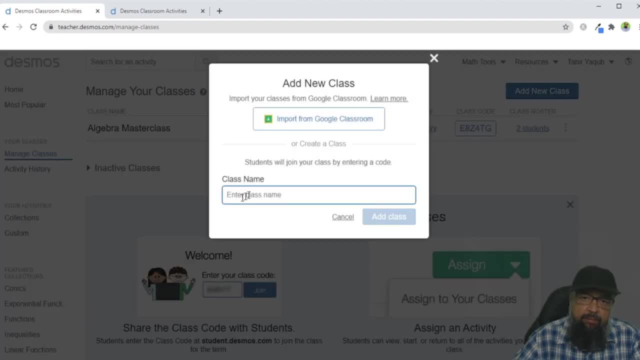 create a new class, simply click on Add new class. you can also import a class from Google Classroom, which is a learning management system, And I will make a separate video on Google Classroom integration with Desmos. give it a name, So let us call it trigonometric class for year. 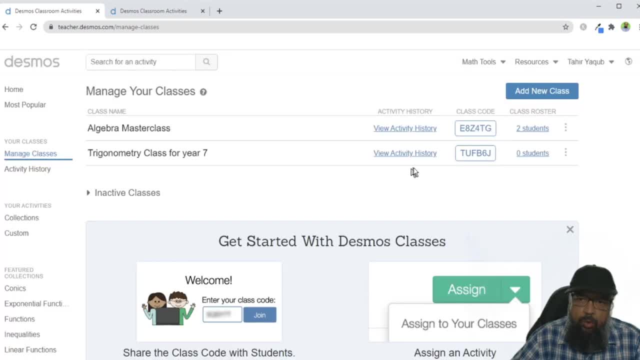 seven, And now I click Add class. Now a new class has been created, And if you want to delete this class, you simply click on these three dots and click on deactivate class. class will be deactivated. in this way, You can edit class name. 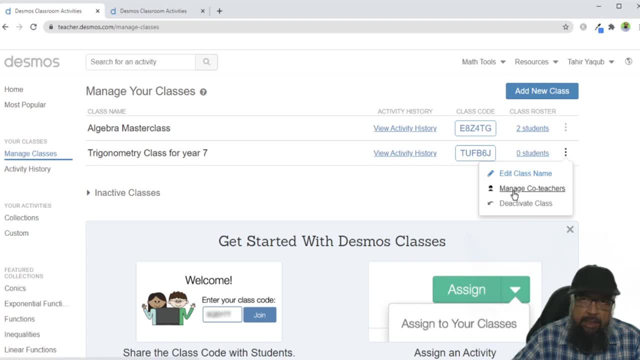 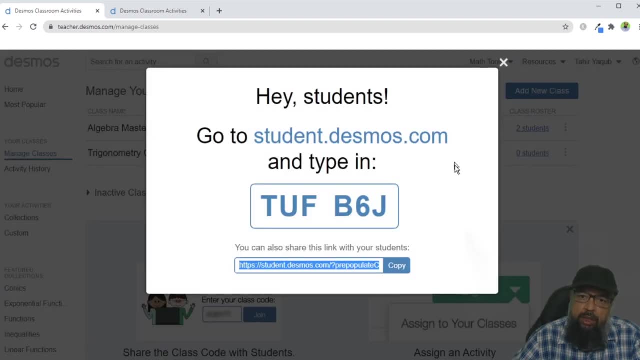 and you can also manage core teachers. by clicking here And now, you will send this link to your students. If you click on this link, it will be shown in large fonts. If you have a whiteboard, you can show this to your students and they will have to log into this web address: student dot. 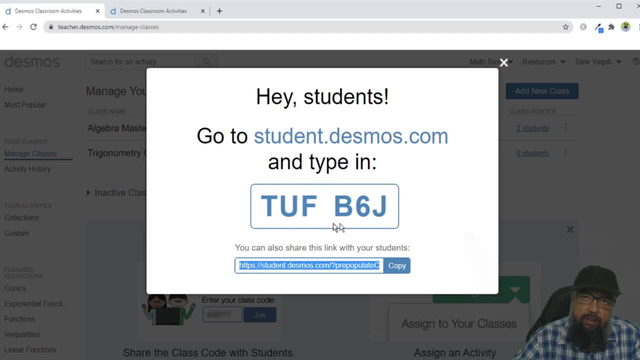 Desmos dot com And there will be a place for class code. they will simply put this class code and then there will be a join button. they click on join and they will be joining the class. Another way is to send this link. I can copy this link. Now. the link is copied. 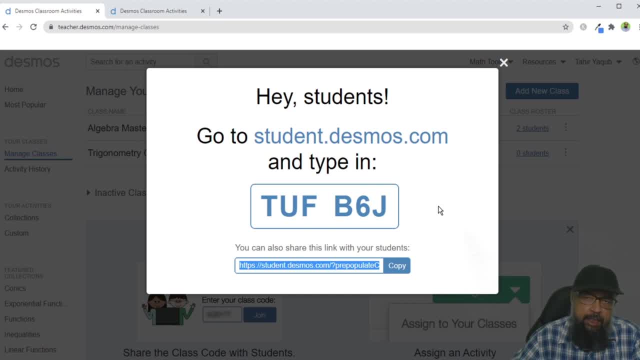 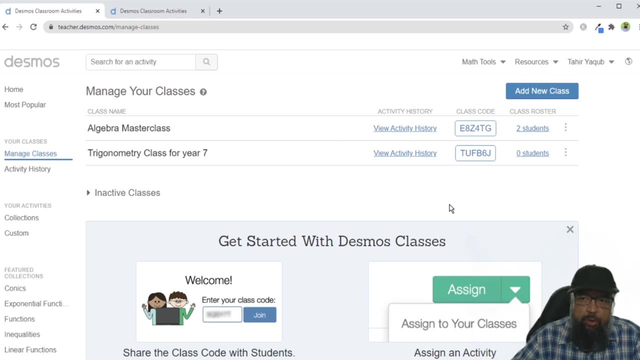 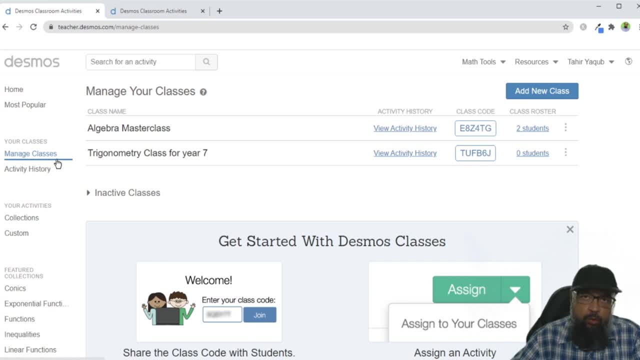 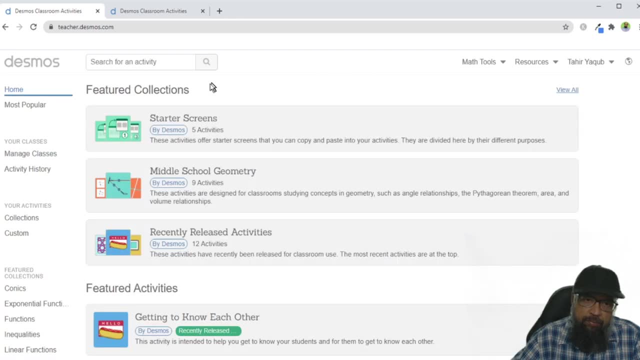 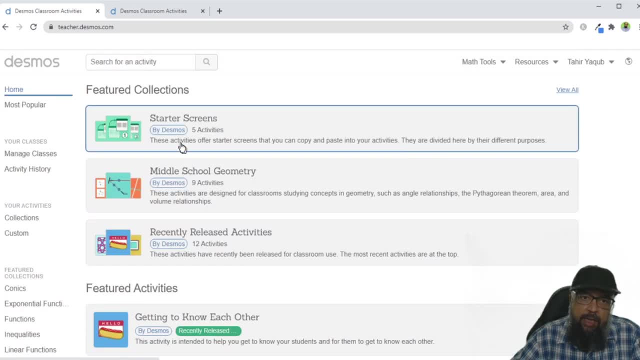 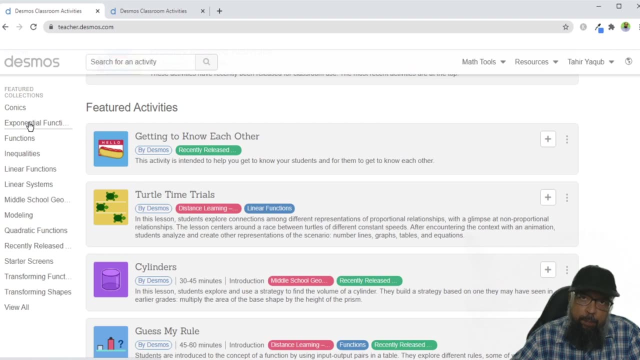 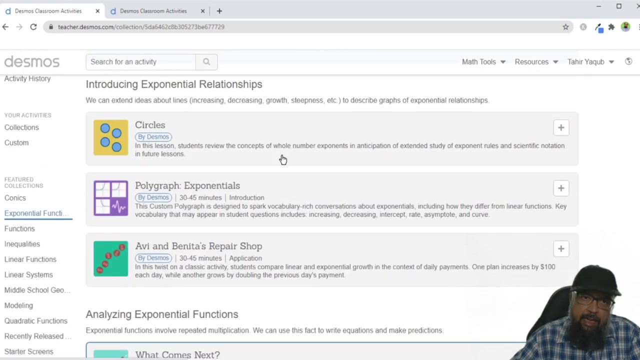 there are some recently released activities. you can also create your own collections around any particular topic, And on the left hand side you will see some math topics And if I click on any of these topics, there are activities arranged within that topic, And then what you do is you when you find any activity. 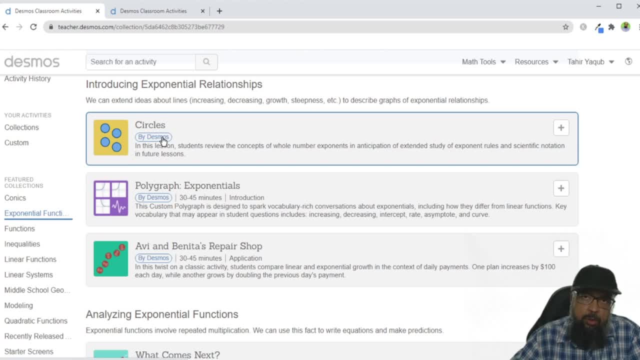 then you assign this activity to any of your classes. So let us first find an activity, And I am going to give you a very simple example which is easy to demonstrate, because some activities are more involving And those will make this video very long. 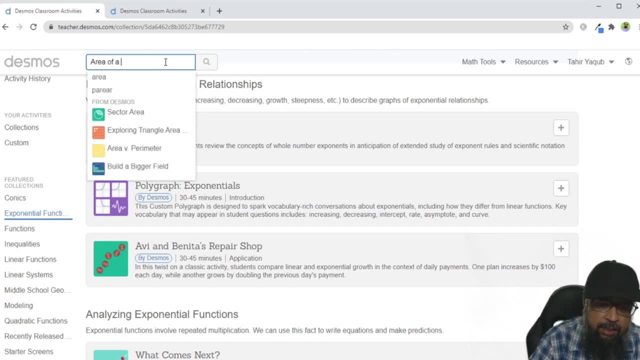 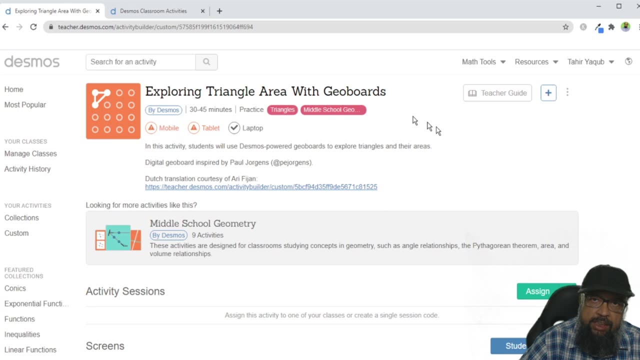 I put something area of a triangle And now I find this activity explaining triangle area. So I click on that And now this is the activity page. Now the first thing you should do is click on teachers guide, because it will help you conduct this activity in your 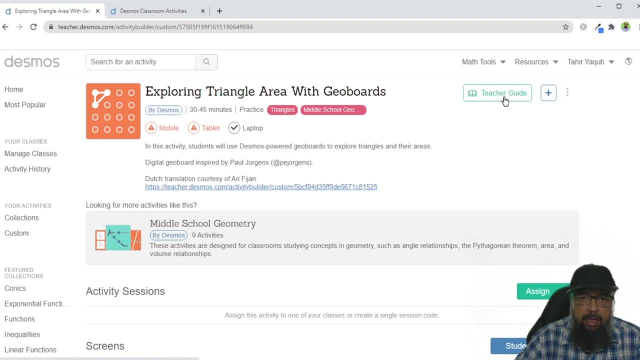 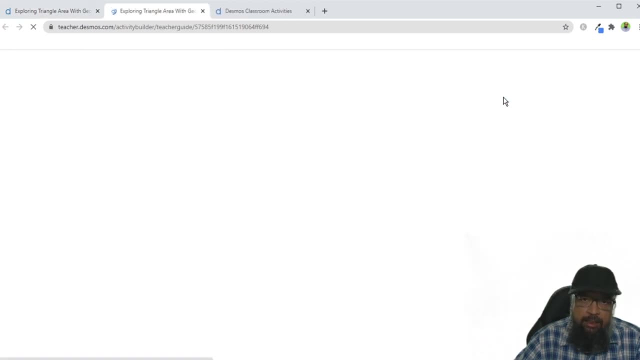 math class, And the first thing you should understand is that the purpose of all this exercise is that your students must learn something. So if I click on this teacher's guide, there are some instructions about this activity And they recommend that you print this teacher's 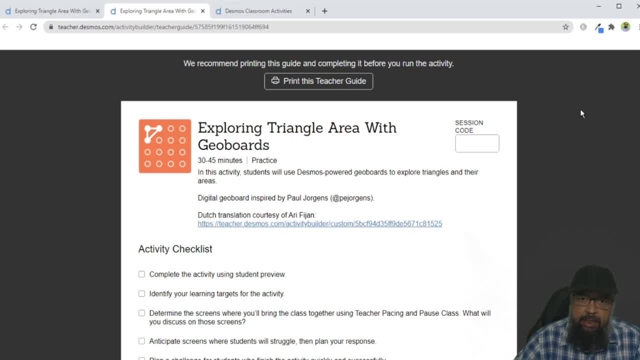 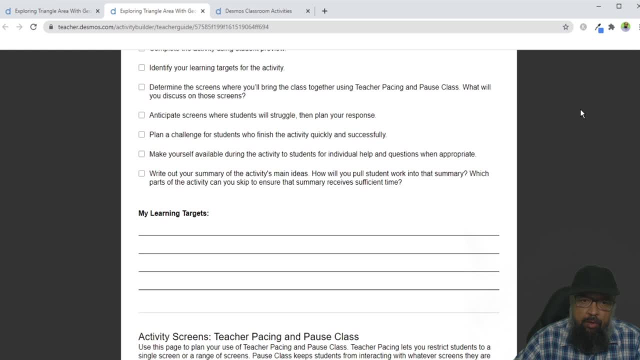 guide and you read it before you conduct the activity, because the designer of the activity wants to show you how you should be conducting this activity in your math class, For example, what are your learning targets? So there is some explanation you should read from here. 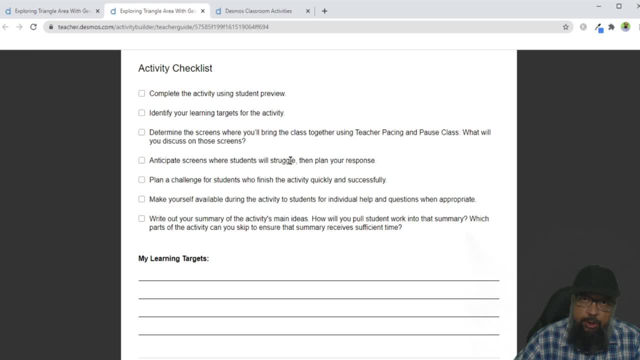 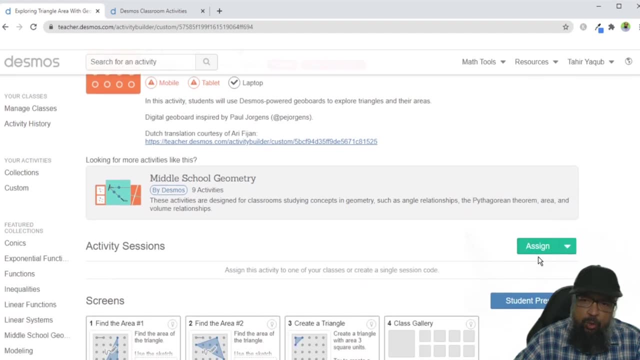 because I have already read this. So I will not be wasting your time And I will show you how we are going to conduct this activity. So I'm closing this. So the first thing you should do is you click on this assign, And then you will be given a manual. So you will be given a manual. 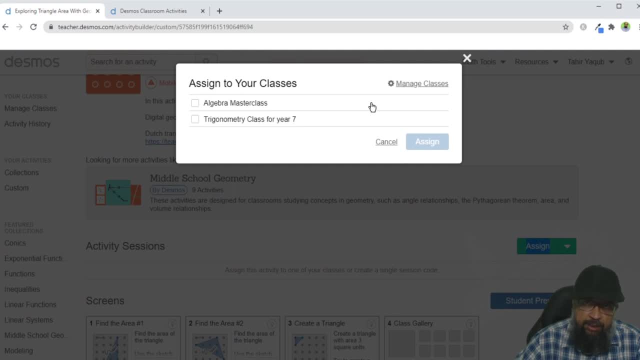 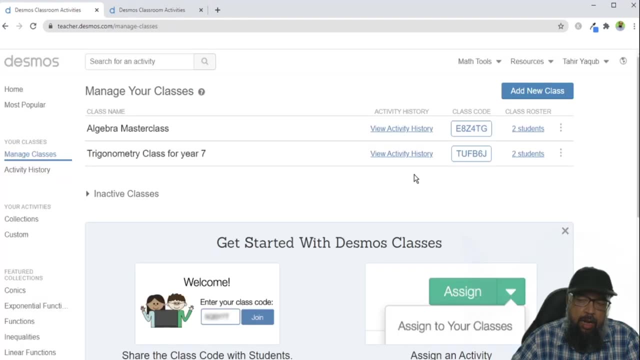 And then you will be given a manual, And then you will be given a manual, And then you will be given and which class you want to assign this activity. So let us assign this to technometric class And I select this class and I click assign. And now I have logged into student Desmos. 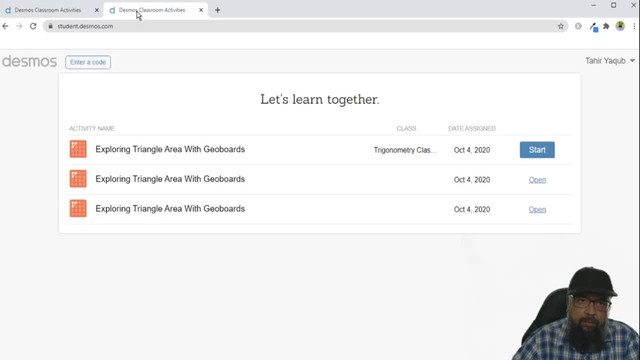 area by using two other devices And if I click on this tab, this is the area where I am logged in as a student And these two are the previously done activities And this is the new activity which I have just received from my teacher And now I can click. 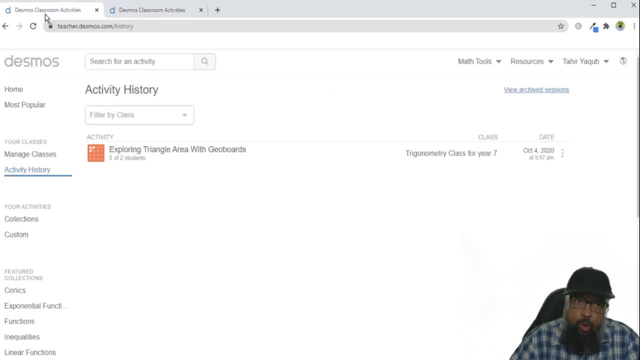 on this start and I can start doing the activity. So in this tab I am in my teachers account And in this activity history menu I can see this recent activity which I have just assigned to my students. I can click on that And this is: 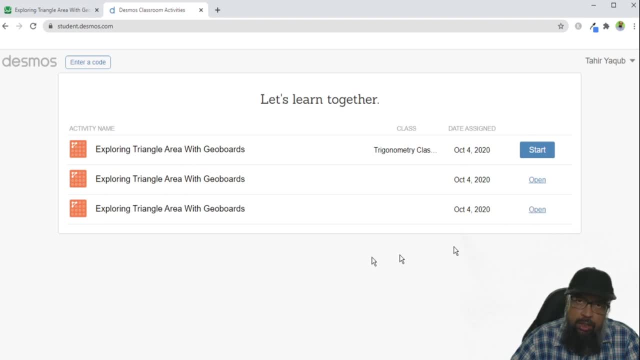 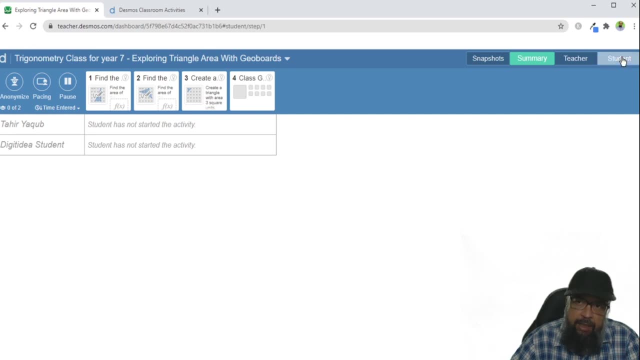 the teachers area. Now, on the right tab, I am logged in as a student. In the left tab, I am using this as a teacher. you can also see the student perspective by clicking on this tab. And now I can click on this activity And. 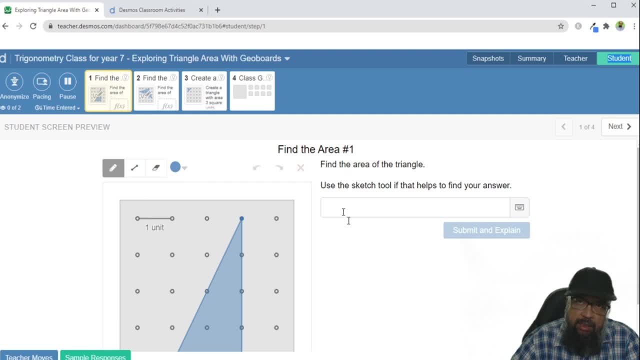 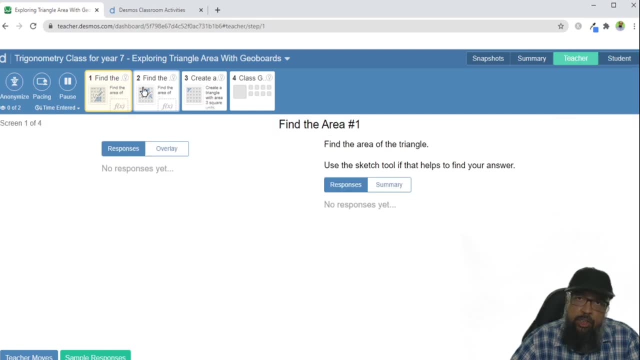 now I can click on this student And you will be able to see how the student will see the activity once the student have started doing the activity. And now let us first see what are these controls? On the left hand side, I have anonymize, anonymize. 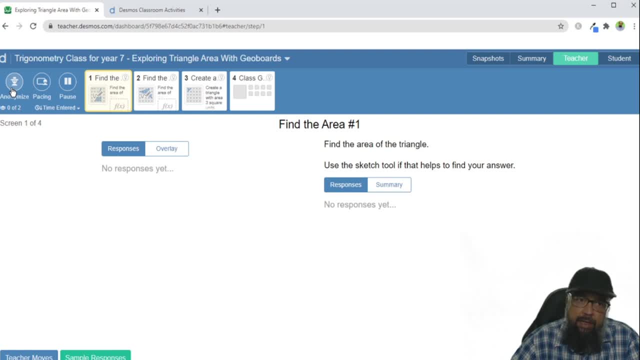 means that if I click on anonymize, I will not be able to see the original names of the students and students will get some anonymous names. So the benefit is that when all students have some randomized names, they will not be get embarrassed if they do something. 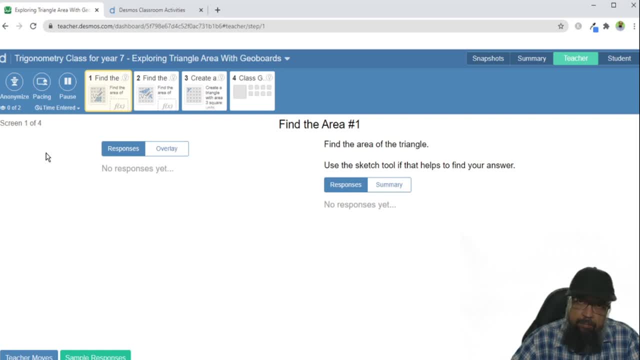 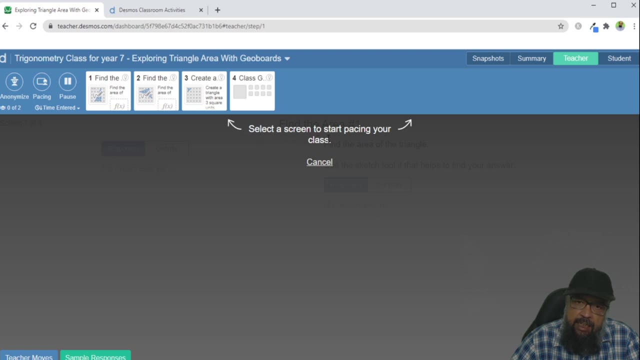 wrong because no one will be able to recognize them. So it is good that you anonymize the students. then is the pacing, And pacing means that how you want to control the activity. So if I click on pacing, you will see this screen. select a screen. 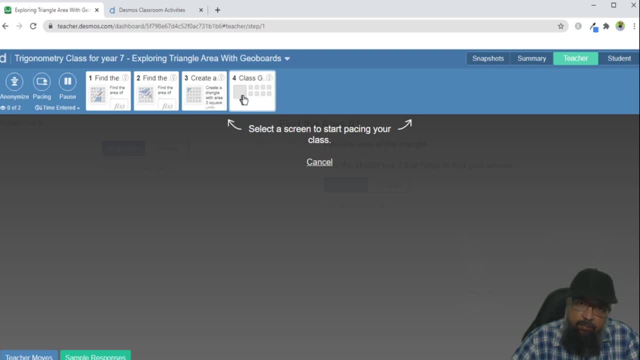 to start pacing your class. So these are four different screens in this activity And I will shortly start the activity as a student and you will see that there are four screens, So when you are pacing you can restrict students to any particular screen. For example, if I click. 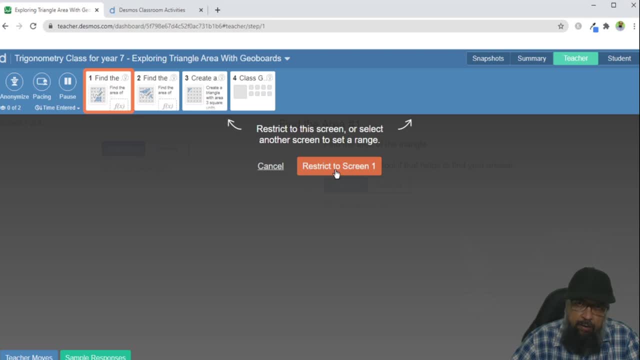 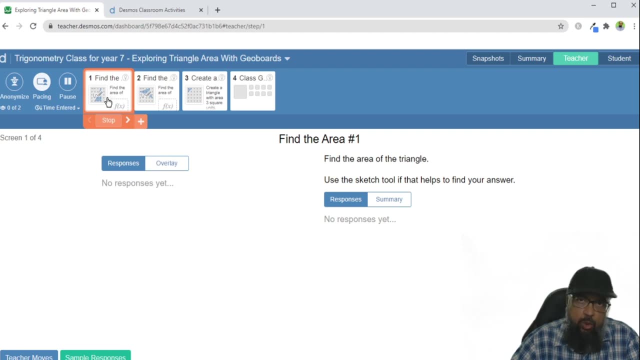 here I can restrict students to screen one if I want. if I click here, students will be restricted to screen one. So if you are in a synchronous online math class, you can restrict your students to this particular screen. then you can move this. 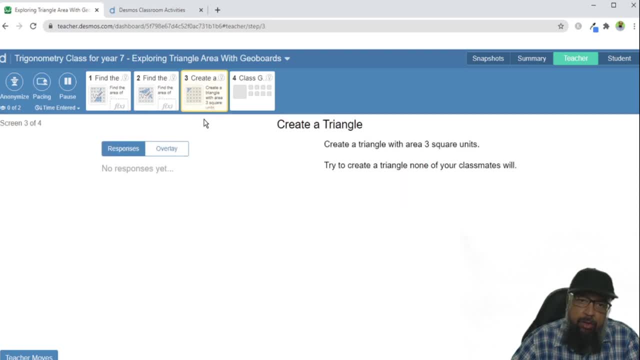 to next and so on, And if you click on stop now you have basically stopped restricting them And if you want to pause the activity altogether, you can click on pause and it will show like this and know if the students want to start the activity, For example. 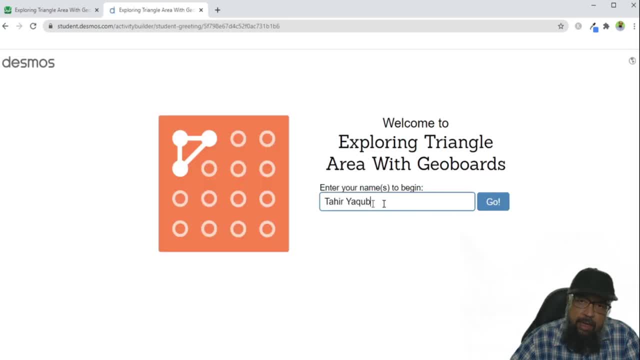 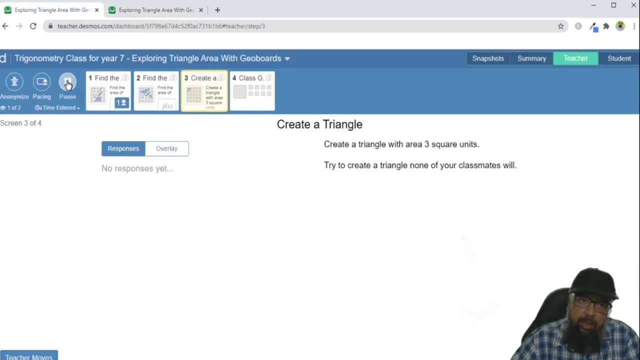 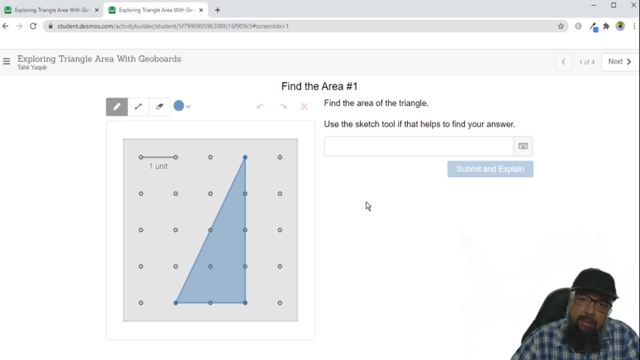 if I go back and I want to start this activity and I give my name and I click Go, I will see this message: that activity passed And now I can click on this pause once again, This green background will clear And now, as a student, I 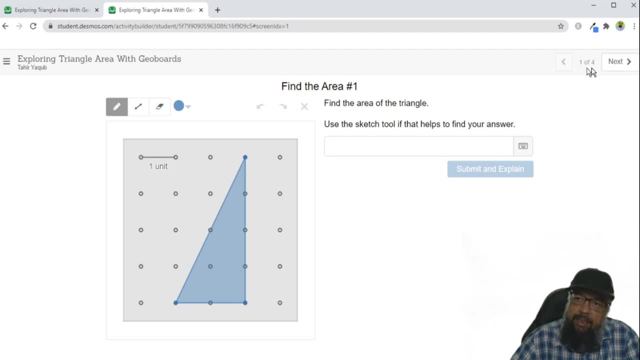 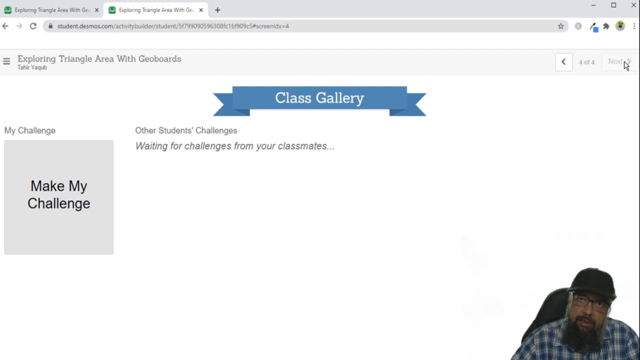 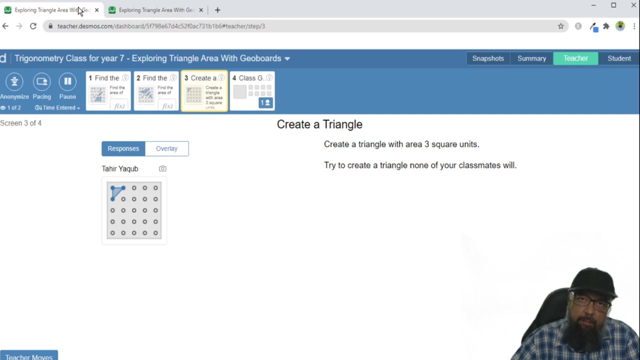 am able to start the activity on this activity. On the right hand side there are four screens and I can scroll and move to the next screen because teacher is not restricting me at the moment. So there are some situations where you want to restrict students to one screen at a time. before you reveal the 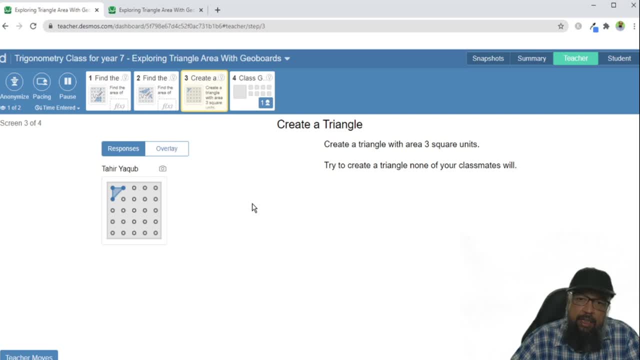 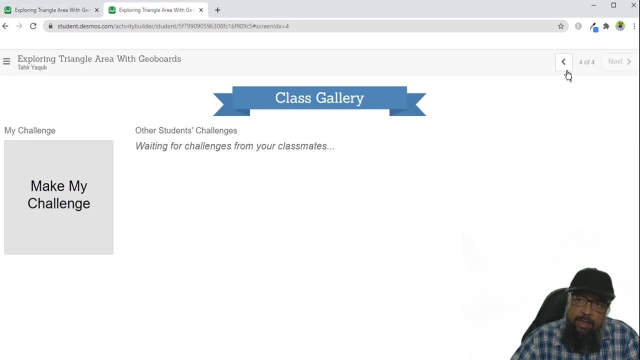 next one. And now, what is this activity? let's have a look at the activity and try to understand what are the things students are learning in this activity. So let us go back to screen one, although the purpose of this video is not to teach you mathematics, but I want to show. 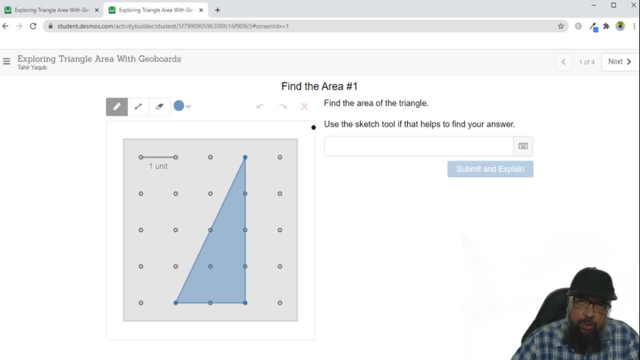 you this so that you can design your own activities later on. Now the activity says: find the area of the triangle, use the sketch tool. These are sketch tools, if that helped to find the answer. And now let's say I typed the area of the triangle. 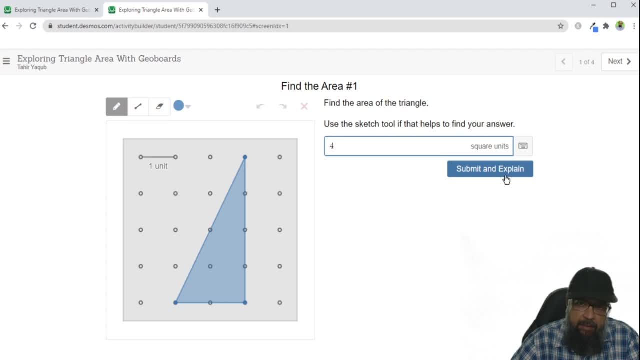 as four. then it says submit and explain. So I can now submit and then there will be an explanation box and I can explain something here. For example, I can say that I use this sketch tool, I draw a line, something like this I made. 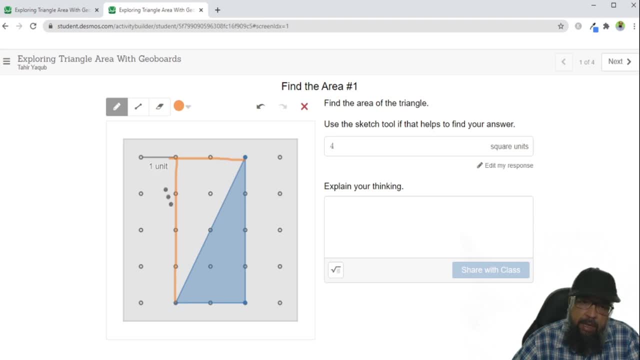 this a rectangle, and the area of the rectangle is two. multiplied by four is eight And this triangle is half of that. So I can explain like this that the area of the rectangle rectangle is eight, triangle is half of that, So it is four. And I click on share with class And then I move. 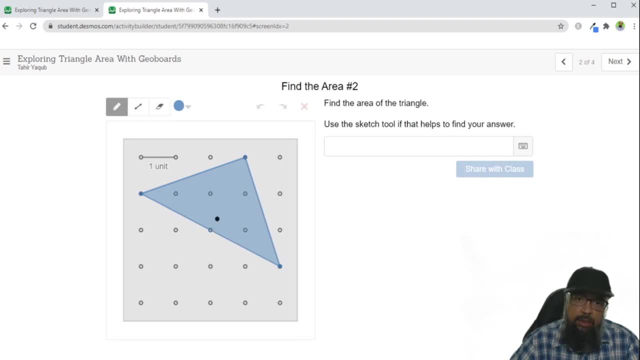 on to the next screen And on this screen. I know that this is a challenging task for students, So if I know this thing in advance, I can look at their responses and I can see what are the issues, why they are not learning what action should be. 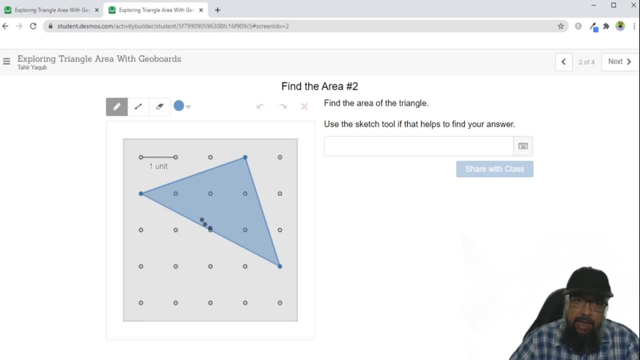 taken as a teacher so that they should learn something, because here they have to use these tools, Otherwise they won't be able to find the area. they have to construct some triangles. then they will subtract triangle areas from a rectangle area and find the area of this triangle, which is 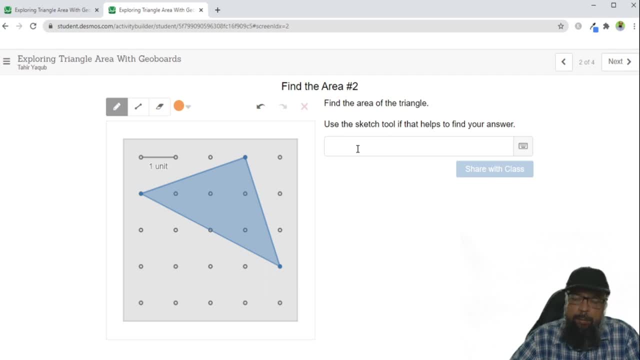 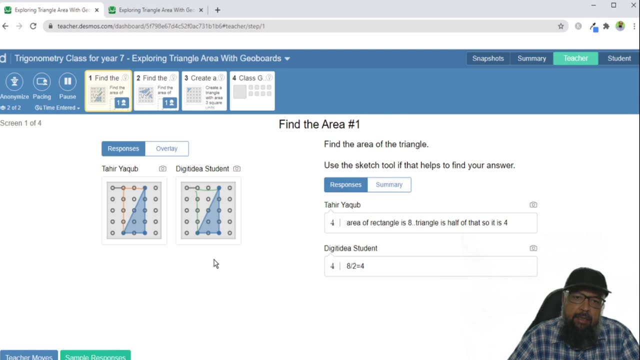 shaded in blue color. So make sure that you are not just copy pasting these activities. the effort should always be to make your students learn something. And now I have submitted the response as a second student from my other device, So for screen one. 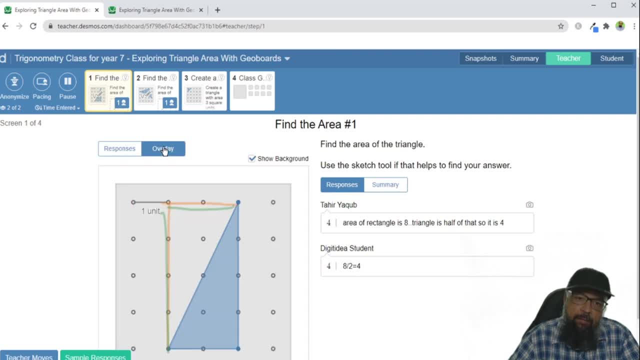 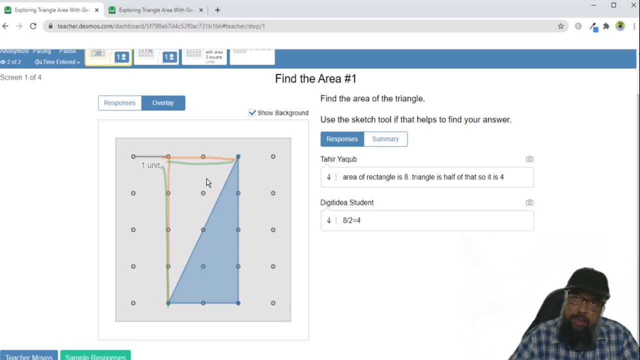 I can see both responses and I can click on overlay And these both responses will be on a single slide Because for some activities this might be important. On the right hand side I can see the explanation of both students. student one: try. 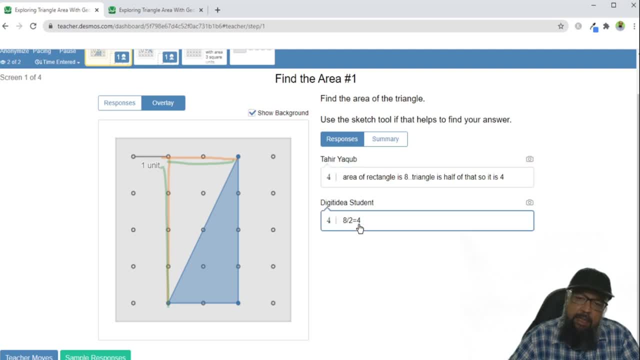 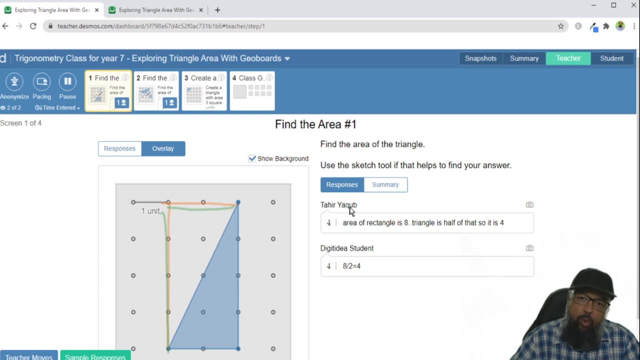 to explain in this manner, student to try to explain in another manner And you can see what approach they are using. And now you can see the original name of the students. These are my names From those accounts, So if I click on anonymize now, you will. 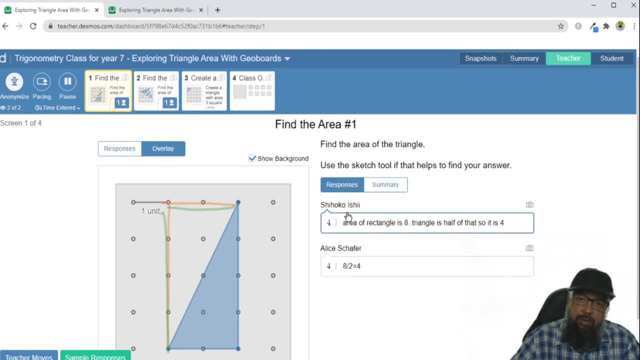 notice that both of these names have changed. Now these are random names assigned by the Desmos application. So in this way you can see the responses of your students, see their answers, what they are doing, how they are doing. So in a 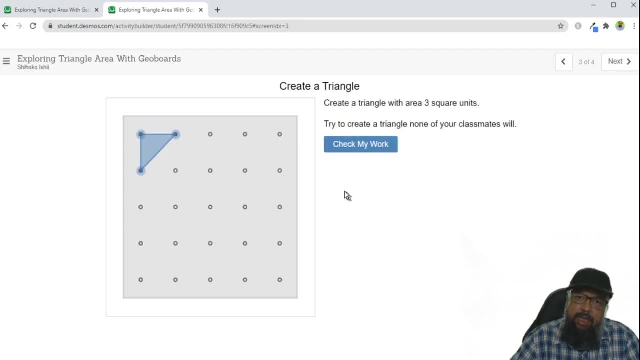 similar way they can solve this question. then in the next question they have to create a triangle which has area equal to three square units, And now, as a student, I can stretch these and then in this direction as well, And now I can calculate that. 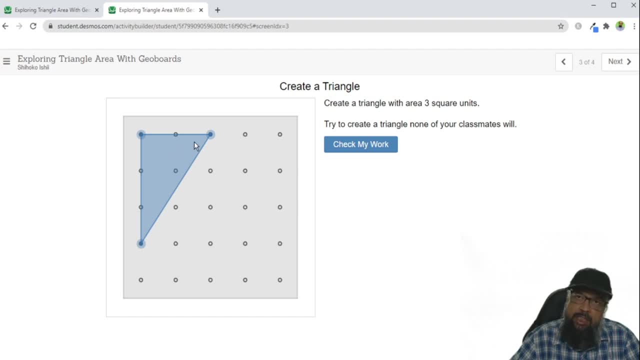 three is the perpendicular and two is the base. three to the six and the area will be half of six, which is three. So I think that this is correct. So what I can do is I can click on this, check my work And I will get. this area is three square. 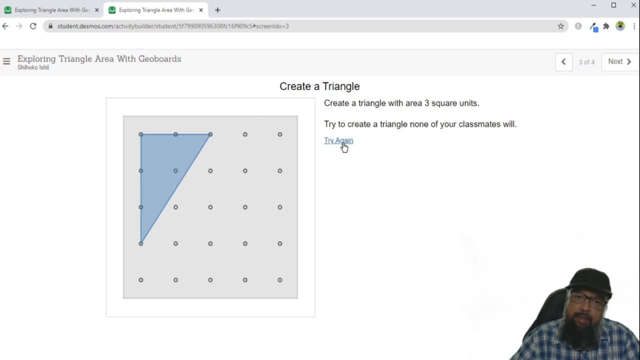 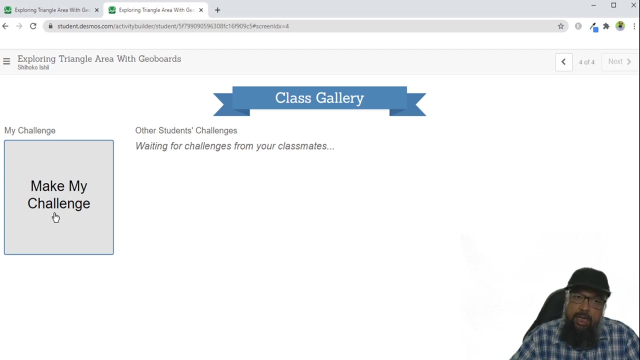 meter And my answer is correct. If, for example, the area is wrong, I can try again. let us go back to the next one, And here I have to create a challenge for my class. So this activity allows you, as a student, to create a similar type of 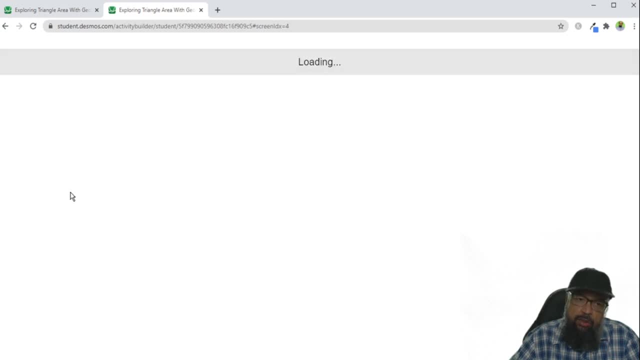 challenge for your class. So how to do that? I click on make my challenge And now it's time to create your own challenge. first, drag the points to create a triangle. So now I have to create a triangle And I will submit meet a correct answer And the application will check that. 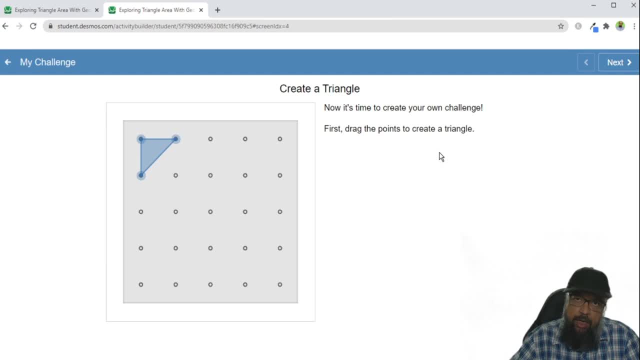 whether I know the correct answer or not. if my answer is correct, then this will be challenged for my colleagues, for my other students. So in this way, all students can create a challenge for other students. So let us create any triangle and move this to the middle, And I can stretch this. And now I know. 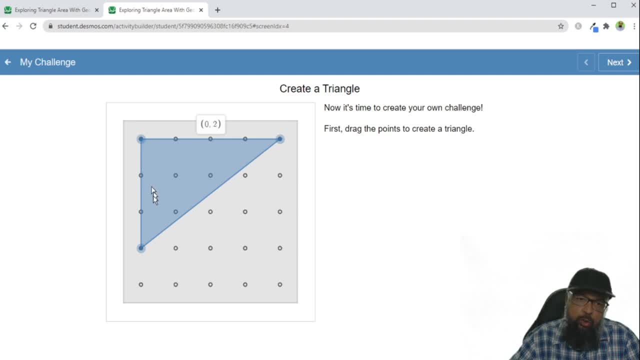 the area of this triangle will be 1234, 123. 12 divided by two is six. Now my triangle is complete. I will click Next. it will ask me find the area of your triangle and I click six and I submit. it will scan and it will see that. 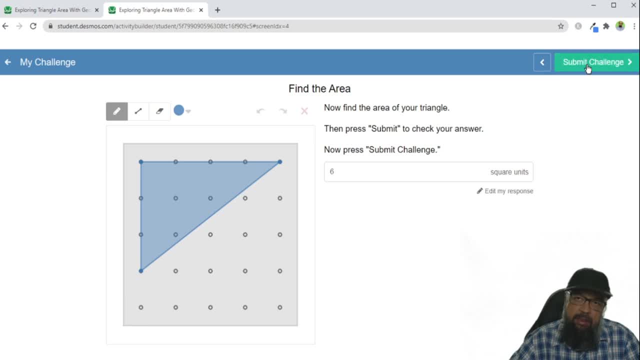 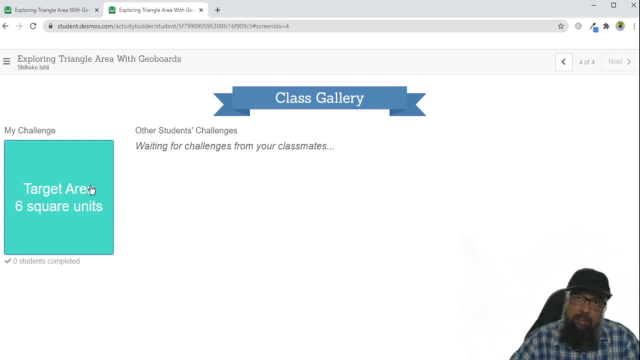 this area is correct. And now I have this button, submit challenge. And if I click on Submit challenge, no, I will see this. This is my challenge for the class And, in the similar manner, every student will create a challenge for rest of the students. And now let's go back to the teacher. 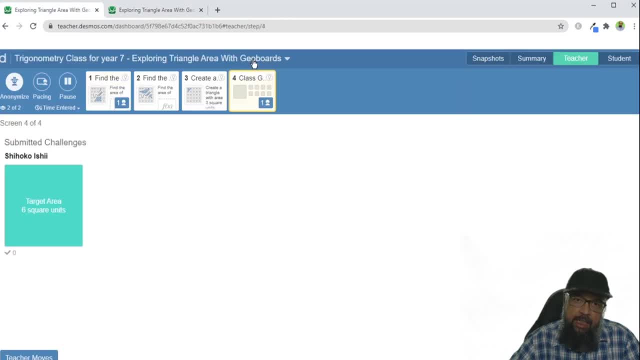 area. And now, if I go to the last slide, I can see that there is one challenge which is created by this student, which is the randomized name. I can see the original name as well, So this is how you can perform math activities while teaching math. 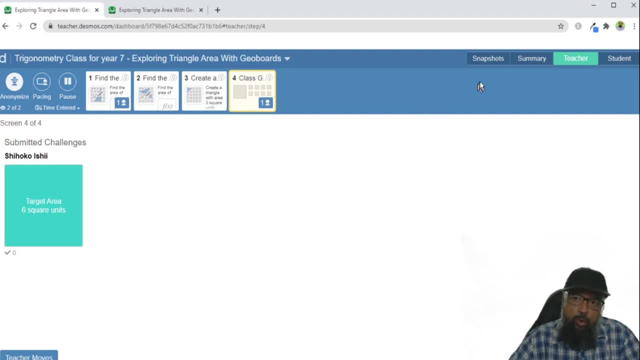 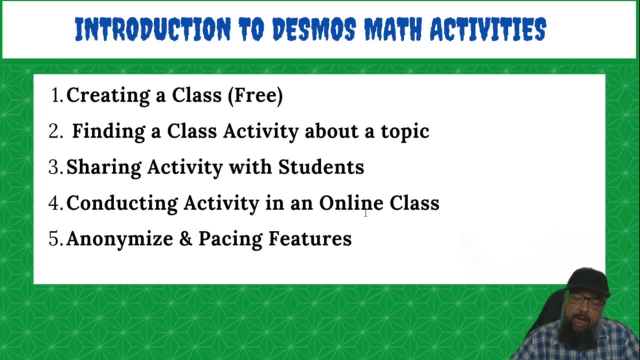 classes online Now. in the next video, I will discuss how you can use this snapshot tool and also how to create your own activity. So I hope you like this video. If so, please give it a thumbs up. Thanks for watching and see you. next time.